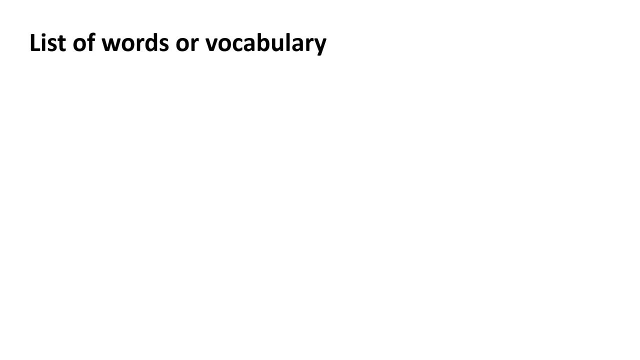 and make a strong vocabulary. Okay, That's, that's one part. Then, once you're done with that, the next thing comes is encoding them. Let me give you an example. Let's say: you haven't you have this kind of data. Uh, we can consider. let's say that it's a training set. Okay, 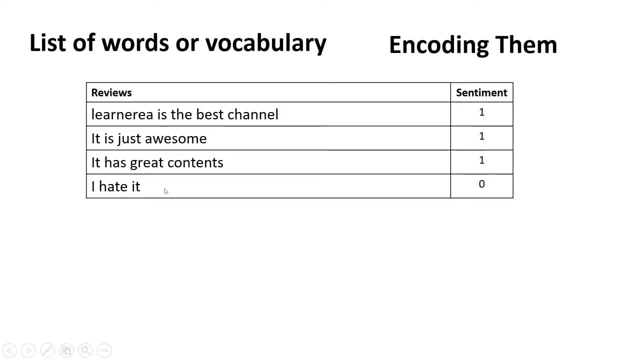 Training data set. So here you see, you have reviews about learn area channel, right. So here it says: learn area is the best channel, It is just awesome, It has great content. And the last review is something someone says I just hate it, Right. So here is the analysis: sentiment analysis. 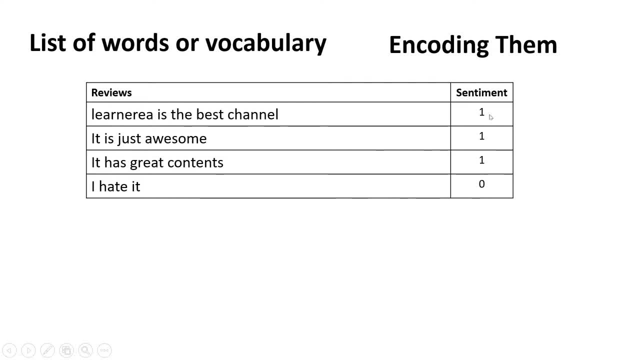 which has been done on this Sentences right. So this in in in terms of machine land learning or, you know, machine learning language or modeling language, we usually say: this is the target variable. This is target variable, which we generally refer as Y, And this is your independent feature. 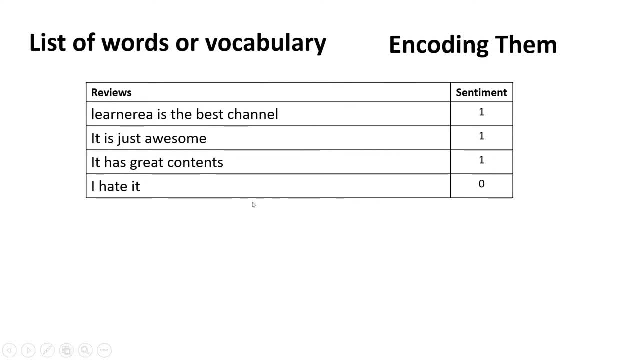 which we generally refer as X. So, using this, we have to train the model to give the result something like this. So how we go? we're going to work on this right. So how does how? how? what is it that we're going to do in bag? 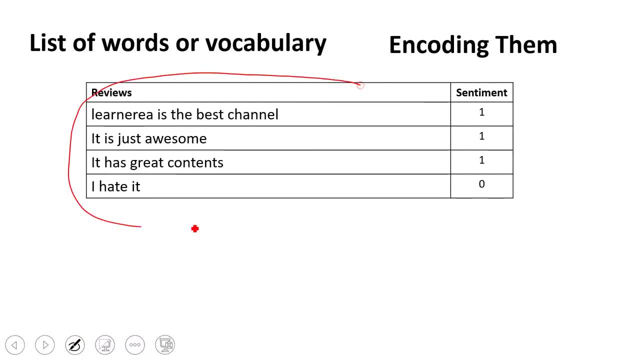 of words, modeling right. So in that, what we do is we have a look at whole sentences, whatever the raw data is being supplied, and then we break them to this smallest unit. You remember we learned in the previous video where we saw how to do the tokenization, So that's exactly what we're going. 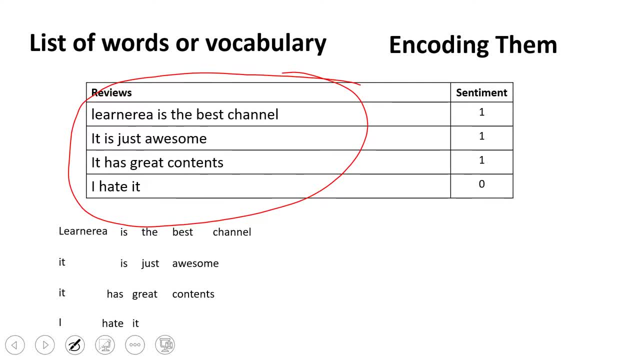 to do over here. So, like you can see, we have broken them to the smallest unit, which is words. right, Of course, words is not the smallest one, Letter is the smallest one, but letter will not make sense, right, In terms of this bag of. 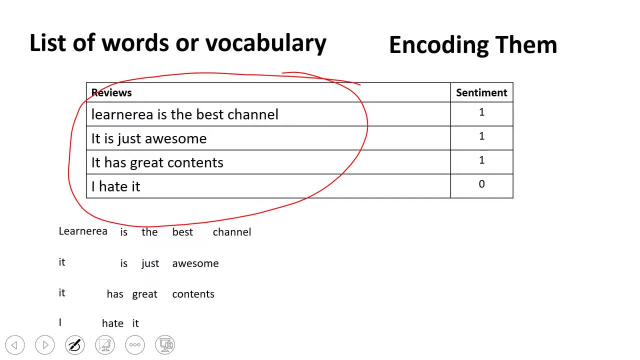 word or NLP language, you will consider that word is the smallest unit. Okay, So now, once you're done with you know, tokenizing all the sentences, all the texts which has been supplied, the next thing which comes is: you know. next thing which I will do is: 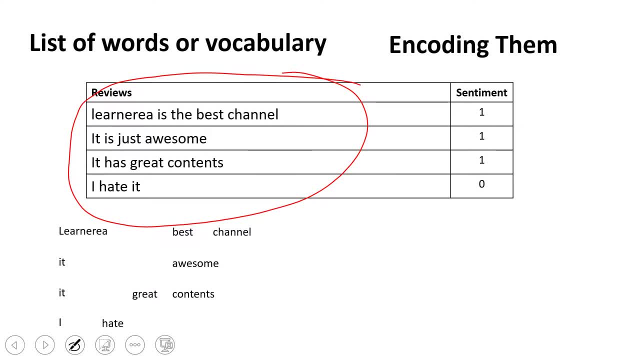 I will remove the stop words. Again, this is something which I have covered in the previous videos. I would highly recommend you to check out the playlist and or I'm I'll be giving the link of the video in the description section. Okay, Now I remove. I'm done with removing the stop. 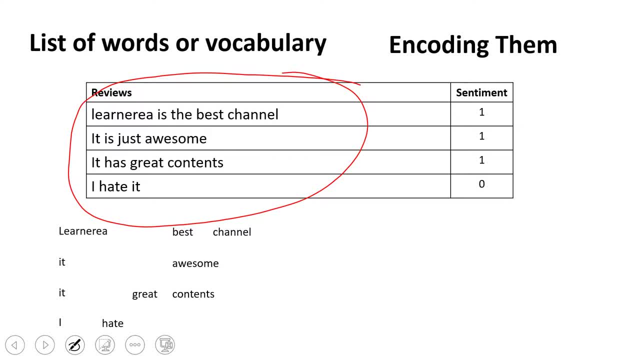 words right, And then the thing comes: is there anything else that we can filter out of it? So yeah, there could be certain situation. For example, here the word NLP doesn't make much sense, And sorry, not the NLP means. this particular word, learn area doesn't make much sense. Other. 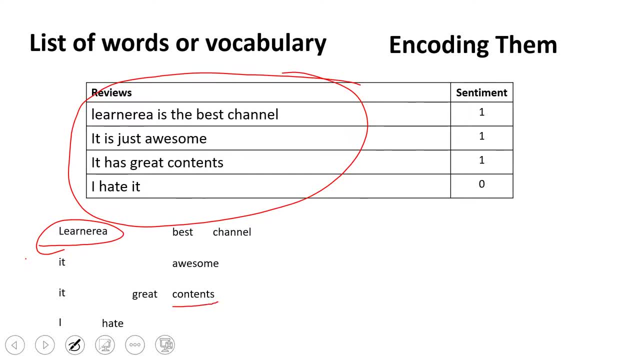 than that we can perform. you know lemmatization or you know stemming, to simplify this kind of words. Other than that, what else that you can perform is? you need to make sure you know how that all the texts are. texts are, in one case, either small or capital. Okay, So that it will. 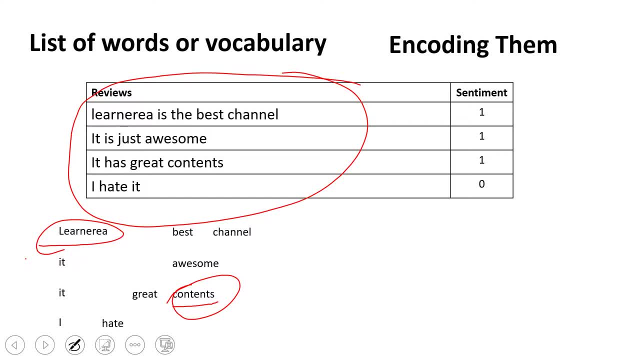 the, the model will not get confused, Otherwise we can start reading the same word as different. Let's say, if you have written learn area in a small letter and in capital letter, both, so that both of them will be treated as separate item. 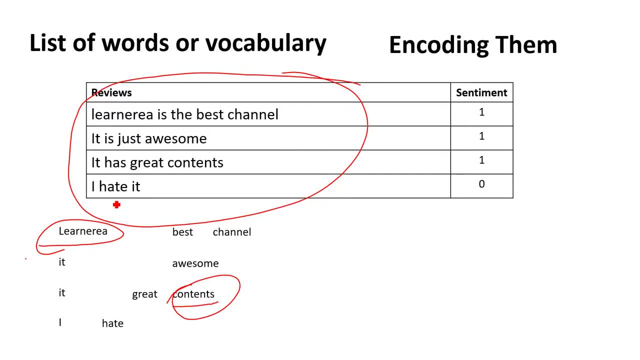 Okay, We will be seeing as we progress in the videos. Okay, How to take care of this, But for now I'm just going to be with these kinds of words. So once we are done with, you know, filtering out this specific word, So this is what our list of words will be, or vocabulary will be. 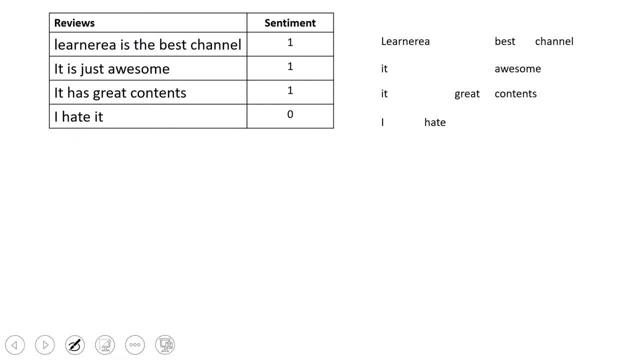 Right. So here to make it clean, I'm keeping it at one side. Now, once we are done with, you know, making all these things, what we're going to do is this: all will be called features. We're going to make them as features, right? So we also say this: feature extraction. Now you can see, learn. 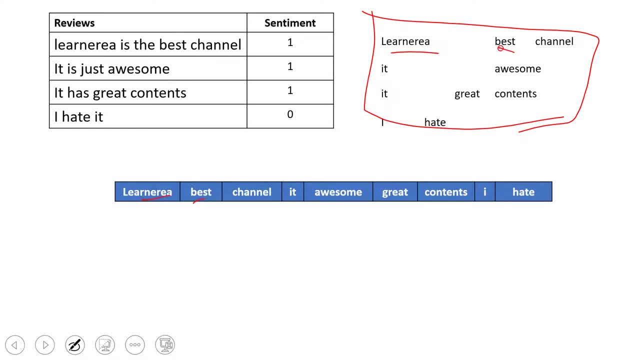 area. This learn area is over here. You know, based is over here. Next thing which we're going to do is we're going to now. once we are done with having all these features created, next thing we will start looking at the supplied sentence. 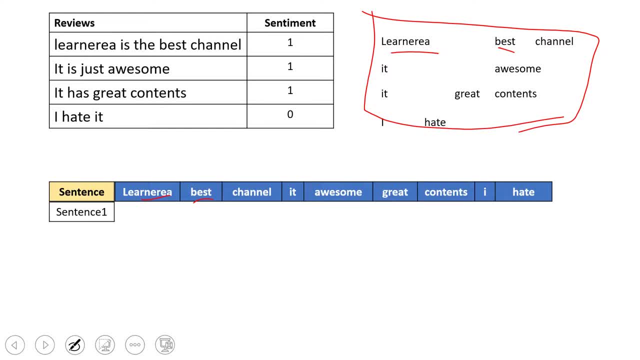 Or documents one by one. So let's pick the sentence number one. So in sentence number one, what you see is: learn area is available, right, Best is available, Channel is available. So when you encode this, So this is what you get: Wherever you find a match, you put one. wherever you don't, 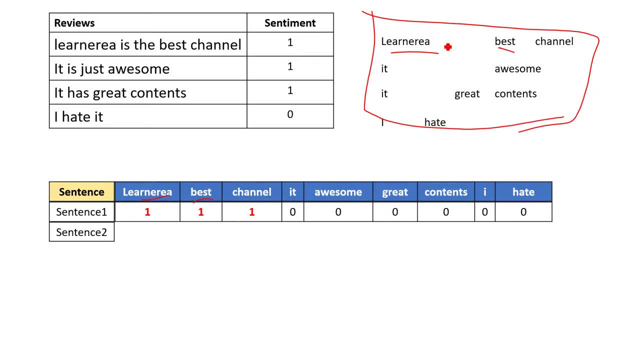 find a match, you put zero. Same thing We're going to do with sentence two, where we see that it has eight and awesome. With sentence three, which has Eight, great and contents. Then we do the same thing with sentence four, where we have I and hate. 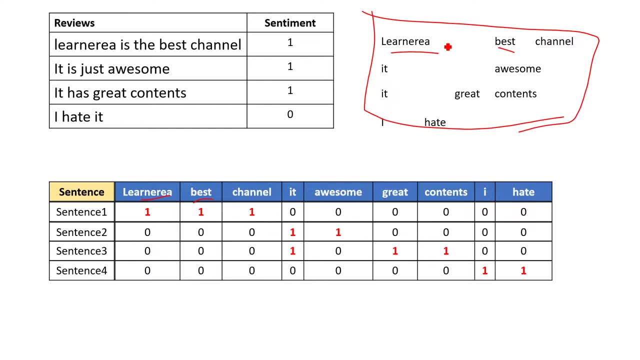 Now this is a very perfect data ready to train your model. Now, when you train the model, so to train the model, you also have to supply the target variable. What is it exactly that we want? So this is the review. So here we are simply saying: if there is any word, if there is any. 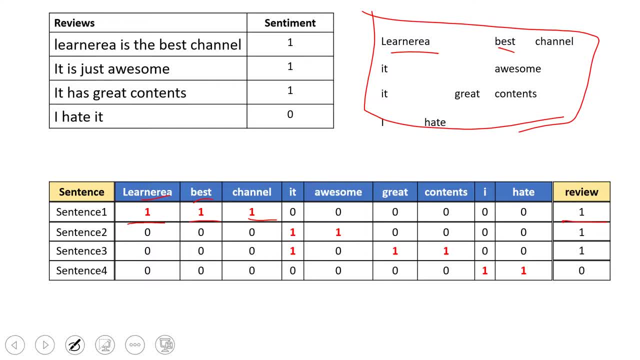 sentence which contains learn area based and channel. That is a positive review. Okay, Same goes for each of the sentences. All right, So using this, you trained your model. Now one thing you should observe over here in the text here: 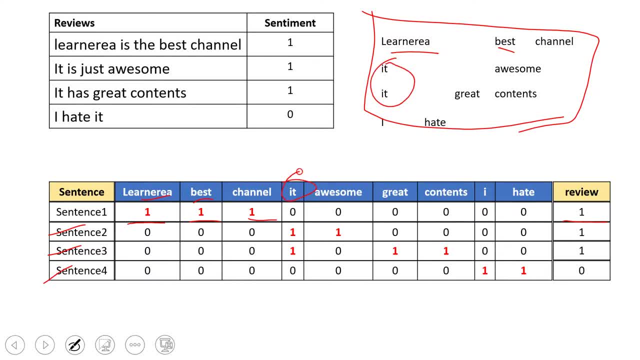 we had to eight word, but here we see only one. that makes sense, right? Because here we are just creating one column and wherever it matches in the sentence we are putting one against that. I just hope that it is clear to you. Now let's take a new sentence where it says: great to learn. 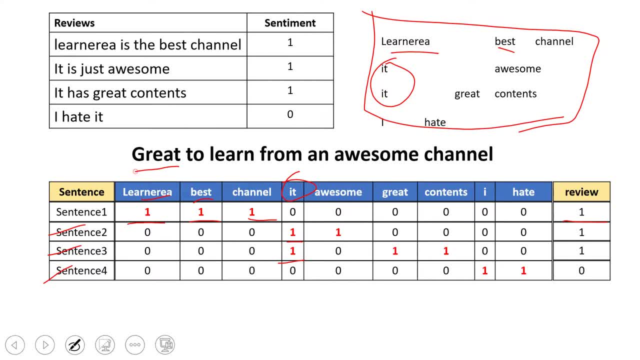 Learn from awesome channel. So you see, there are two things which are matching over here, Three things In fact: great, awesome and channel. Let's put it in this table. So sentence five and that comes something like this: So here you see, channel is something matching. 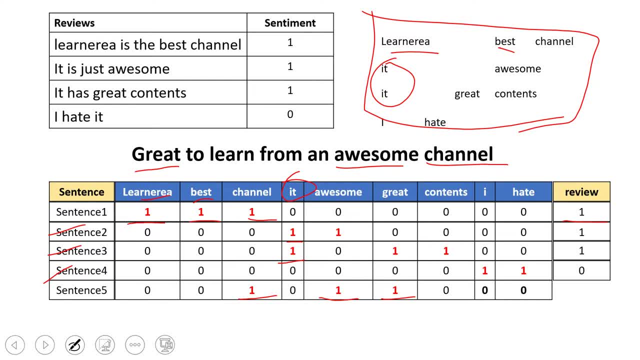 awesome matches and great matches. So we see that these, wherever wherever we had word great, we got a positive review right. Wherever we had awesome, we had a positive review. Wherever we had channel, we also had positive review. Okay. So